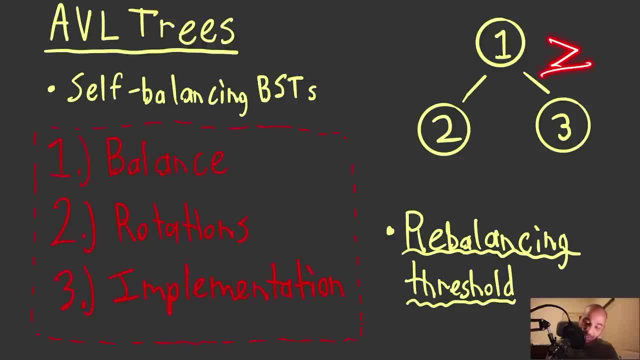 we're going to have items less. If we look in the right subtree, we're going to have items greater than or equal to. Sometimes I've seen it less than or equal to and then greater. All that AVL trees add on to that is we're going to have a self-balancing property to them. 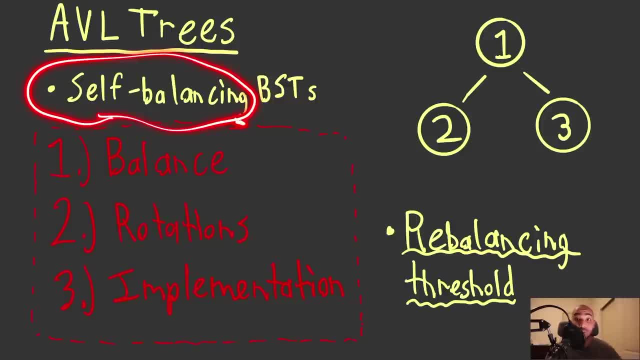 And they're going to balance themselves after we do inserts and after we do deletes. And why do we want to do that? Remember that if we have a binary search tree- let's say we were inserting three, two and one- That is skewed to the left, we see, So that's going to be linear. if we were, 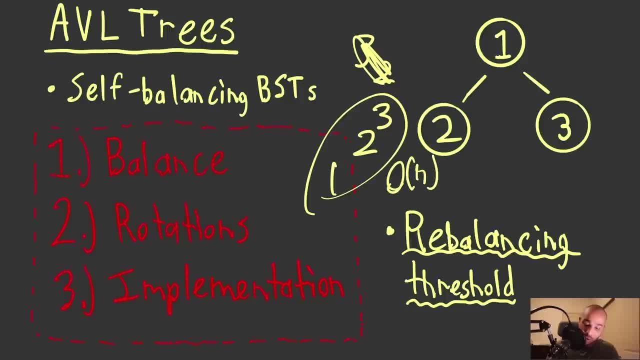 trying to do that. So that's going to be linear. if we were trying to do that, We're going to have to search, because we have three nodes And we're going to have to search all of those nodes. We could go as deep as that last node, The whole thing that we're trying to. 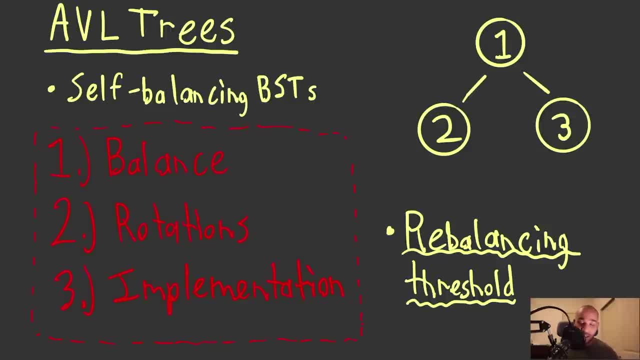 avoid is that skewedness. And if we balance our tree and define certain thresholds on the balance we have at each node, we can keep these searches logarithmic, And that's what we want to do. So that's what we want. We're going to talk about balance. We're going to review what balance is. 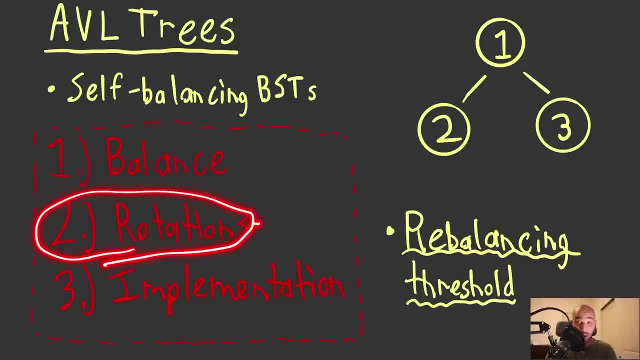 We're going to look at rotation. Where do these rotation operations? We're going to look at left rotations, right rotations, Left, right and right left, And then we're going to be doing an implementation of insertion. In the interest of time, we're just going to do insertion. It's going to be a good bit of code. 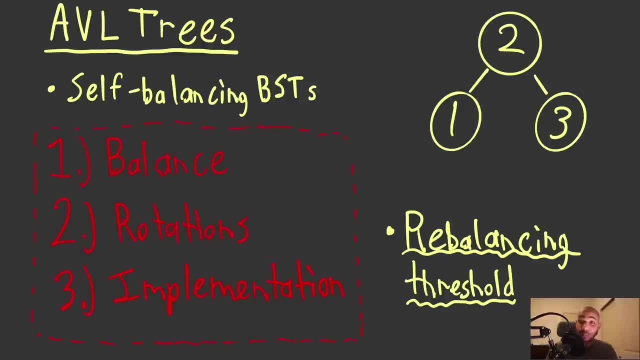 So I just realized that's not a binary search tree. Let me fix that. Going back to that property, we know that our left subtree is less than, and then that right subtree is greater than or equal to, And what we're going to do is we're going to have a rebalancing threshold And we're going to 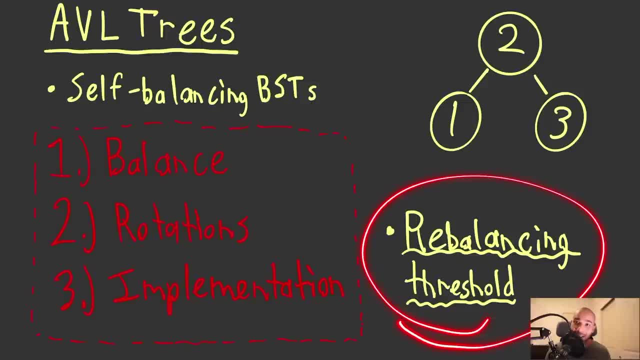 look at the balance at every node in the tree. If we break a certain threshold in standard AVL trees, that's going to be one We're going to need to rebalance. I keep talking about balance thresholds. Let's actually look at the idea of balance first, and then we'll get into our 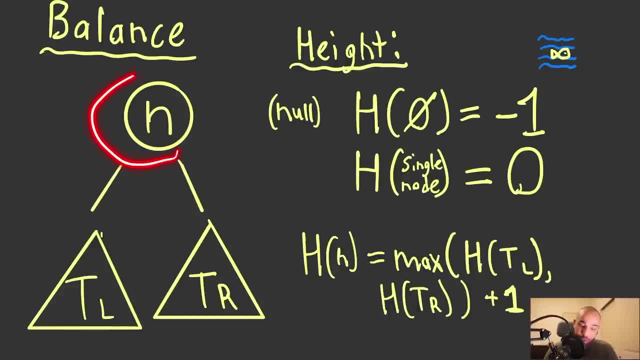 rotations. So now balance. Remember, we always talk about trees in a recursive manner. We have this node N and this node is going to have a left subtree and a right subtree. They're both going to be recursively defined, So every single node roots its own subtree. We think about it. 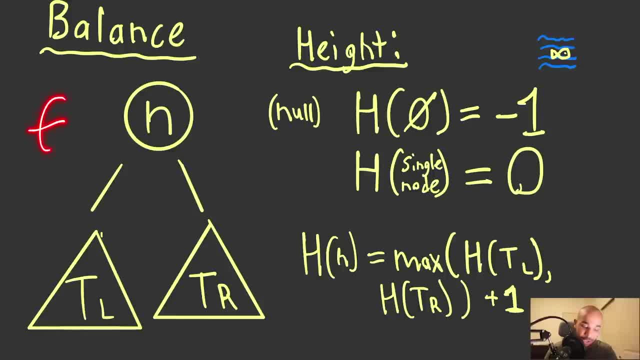 recursively. And if we were thinking in terms of a function, we would have a function and then we would have that node N, And then we would have a left subtree and then we would have a right subtree. We need to define a height. What is the height of a subtree? So if we have nothing, if we just have, 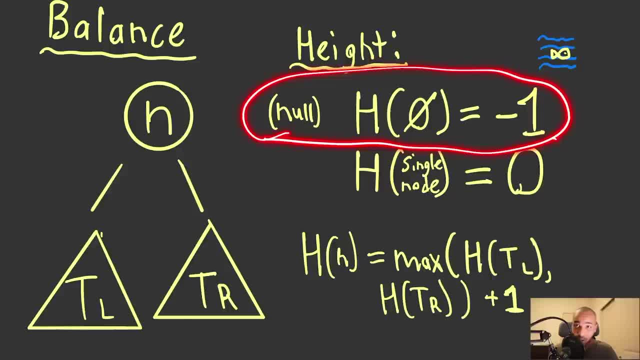 a null node, we're going to say that the height is minus one. We could call it height zero, It could be either, as long as we stay consistent. So we have a height of minus one And I sometimes like to say it's underwater. If we just have a null node, it's like we're underneath the tree, That's. 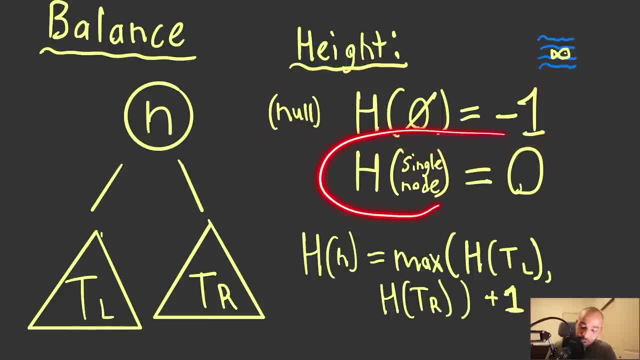 just kind of how I remember it, I have a little fish swimming there And then if we have a single node, we're going to have a height of zero. So in this case, if we just had a single node, that's height zero, And then as soon as we start adding nodes on, we need to have a recursive definition. 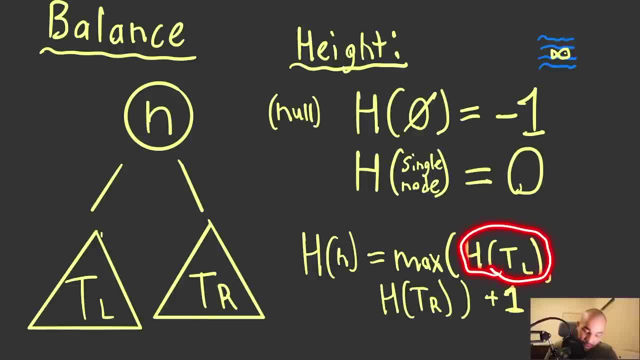 for this height. So we're going to say: let me find the height out of this left subtree, And remember this guy up here that node N wants to know the height of his subtree. The way he's going to get his height is he needs to look at the left subtree he owns and the right subtree. We're going. 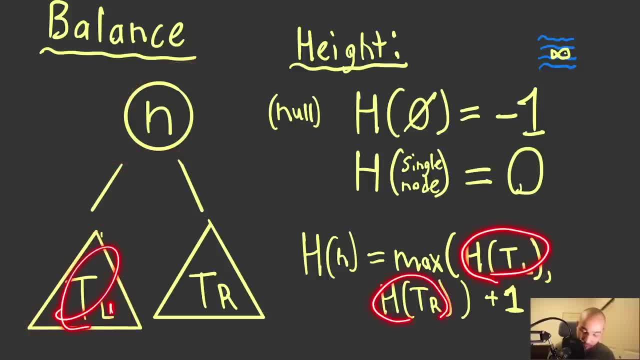 to look at the left subtree right there. We're going to look at the right subtree And then we're going to look at the left subtree right here. We're going to see between these guys who has the larger height, And then we're going to add one to that. So then there we go. That's going to give. 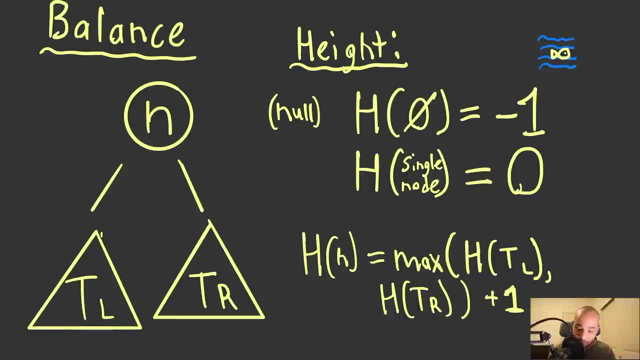 us the height, And we're going to see more examples of this as we continue on. So that is height. If we have nothing, it's going to be minus one. If we have a single node, it's going to be zero. If we 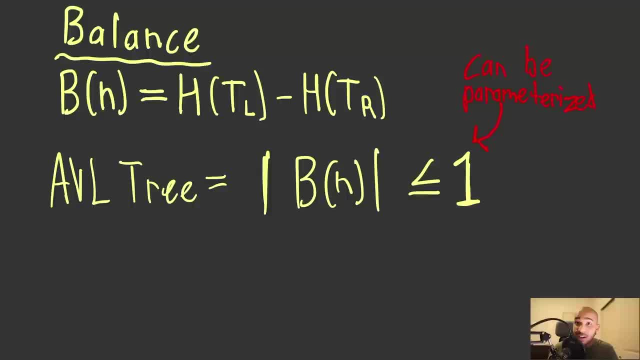 have more than a single node, we're going to need a recursive definition. Now, what is balance at a specific node mean? Balance is going to be the height of the left subtree minus the height of the right subtree. That is going to give us the balance at a certain node, N. And so what an AVL. 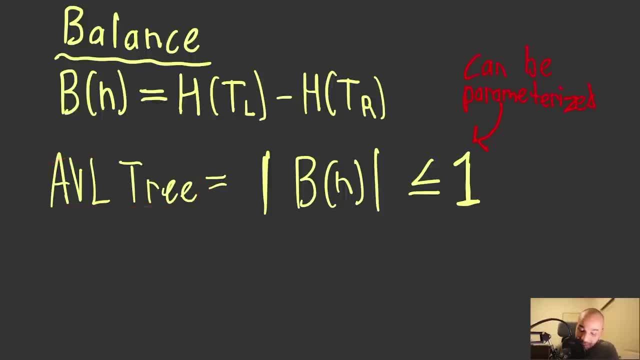 tree does is it's going to keep this balance, the absolute value of this balance, within a certain threshold- And here we see it can be parameterized. So AVL trees are going to have a threshold of one. We can make that threshold more, but the standard threshold is going to be one. So that's what we're. 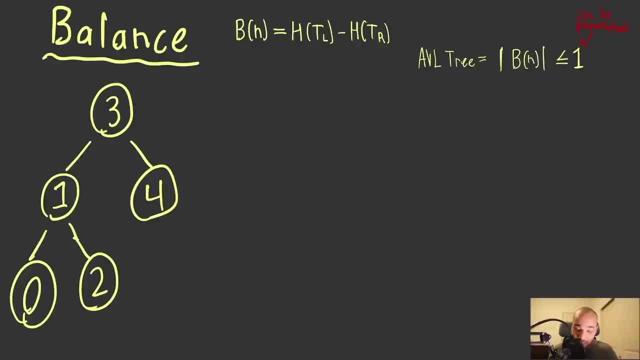 going to see in our examples. Now let's do some examples and start calculating some balance. I've kept these two things up here: our balance equation and how our threshold is going to be one. We're going to start at the root node. What is the balance of that? node three? So we have the balance. 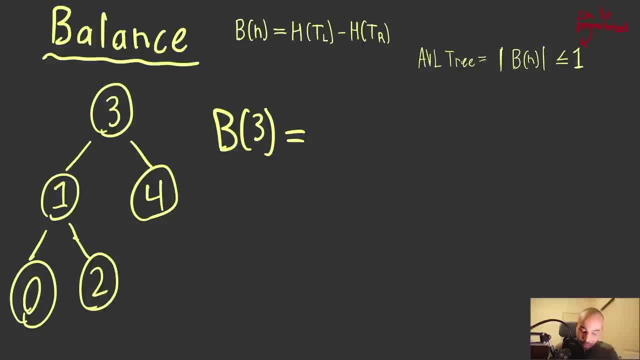 of three. We need to look at the left subtree. So do you see this tree right there? That is a whole tree to itself And we need to consider what the height of that is. So we see a single node at the root. So that's a height of zero, as we defined before. And then we have a left subtree And 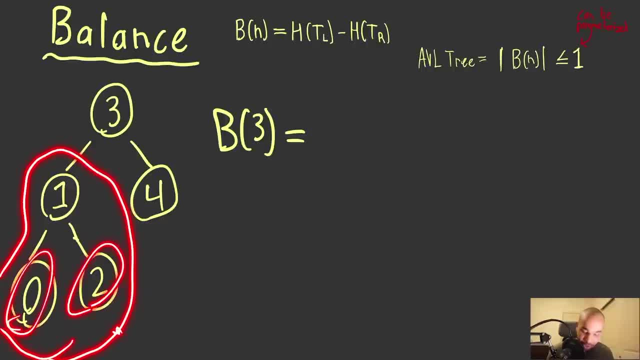 then we have a right subtree, which is just a single node. We have a right subtree, which is just a single node. Ultimately, the height of that left subtree becomes just one, And so the height of that left subtree is one. And now, what is the height of the right subtree That's going to be? 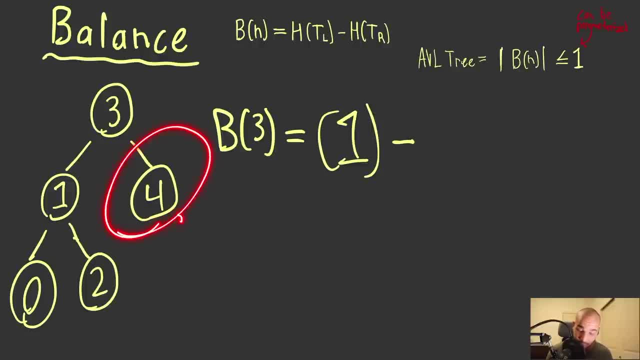 this guy, We see that it's a single node, And since it's a single node, we know that's height zero, And then, once we evaluate this, we're just going to get one. So, okay, now this is one, And 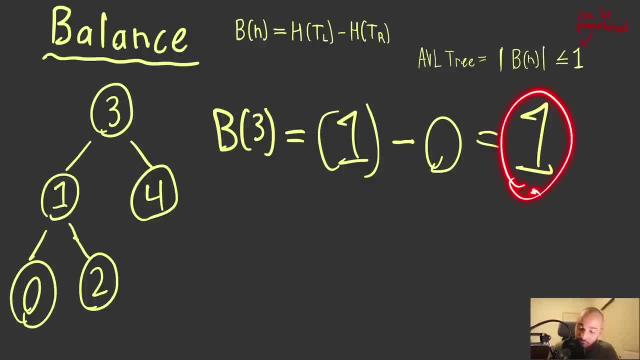 what was our threshold? Our threshold is one. Look at this threshold right there. One is less than or equal to one. One is equal to one. We know that the balance at that top node is one, So let's just make note of that. Okay, So we just 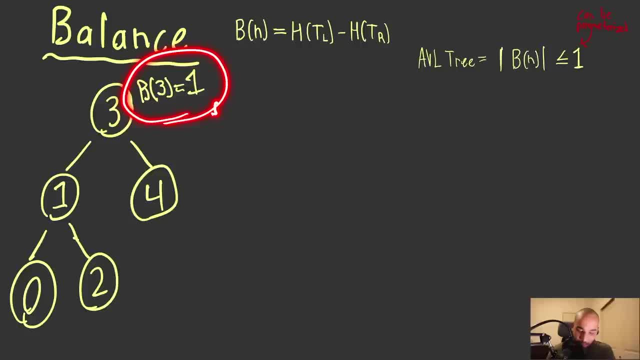 calculated the balance at the root node. The balance is one And I want you to notice something: This is left heavy. So I want you to notice: look at the equation. If we have a positive balance, that means that that left side of the equation, that guy right there, is dominating and he's going. 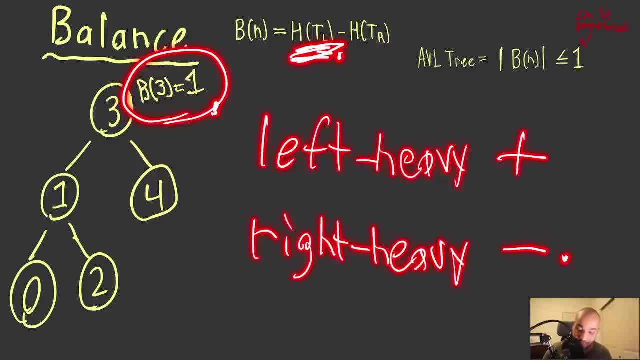 to bring us positive. That means we're left heavy. If we're right heavy, our balance is going to be negative. This guy over here is going to dominate our equation. That is something to just pay attention to. That's going to be a part of our pattern matching. later It'll make 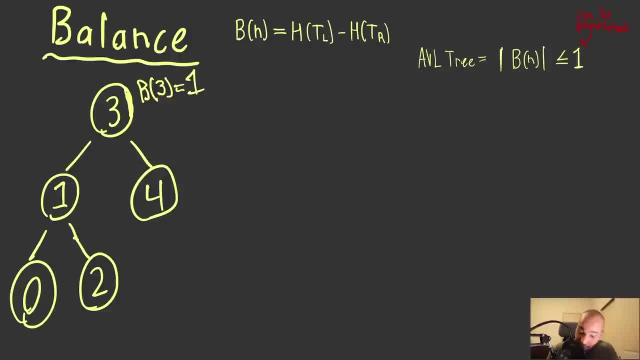 it really easy to internalize our rotations later. So now we can continue on. We can calculate the balance for this guy right here. What is the balance for him? So we're going to say what is the height of his left subtree minus one, What is the height of his right subtree minus one, And then 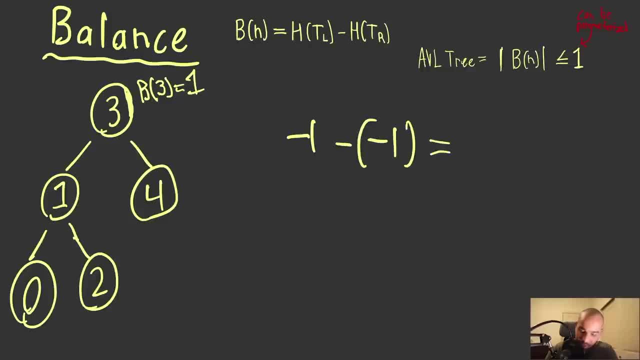 one minus one minus minus one, That's just going to be zero. So the balance at four is zero. Okay, So now let's look at the one. Let's calculate the balance over there: The left subtree, single node- What is a single node? Height zero. And then we need to find the 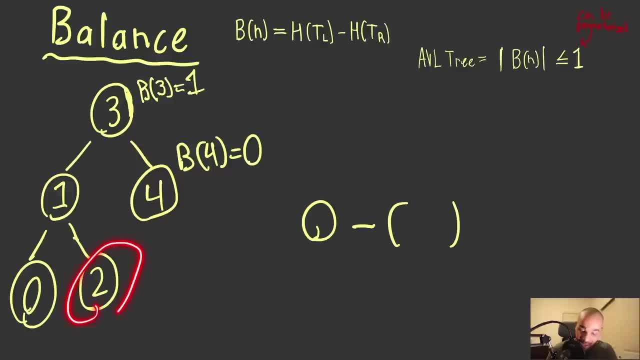 right subtree height. We need to find the height of that guy right there. His height is zero. He's just a single node. So zero minus zero is zero. So that means that the height at this one is going to be zero or the balance is going to be zero, And so if we continue on, we're going to see. 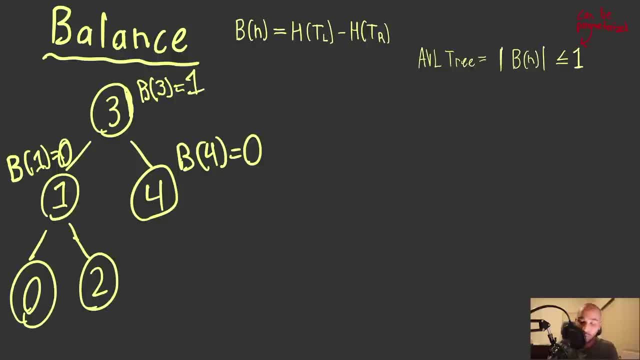 that the balance of this zero here is just zero. He has a minus one left, minus one right. That's just going to become zero. Same thing for that guy right here. So we're going to calculate the right subtree height here. So we're just going to make those zero So we can see that this tree 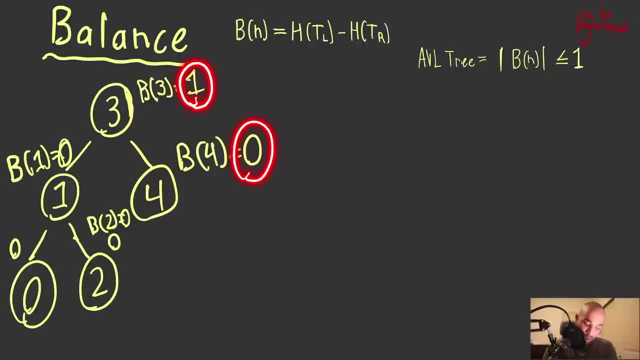 is special. We have a balance of one, balance of zero, balance of zero, balance of zero, a balance of zero. All of those are within our balance parameter. We want to stay within a balance of one, So the absolute value of any of those will be less than or equal to one. This is an AVL tree. 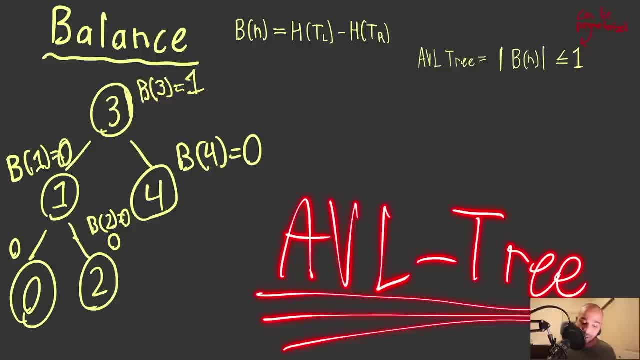 It is adhered to our threshold. All of the balances check out and there's nothing we need to do here. This tree is balanced. We're going to have to do something about it. We're going to have logarithmic search. Now let's look at a tree that might not adhere to this property, So let's. 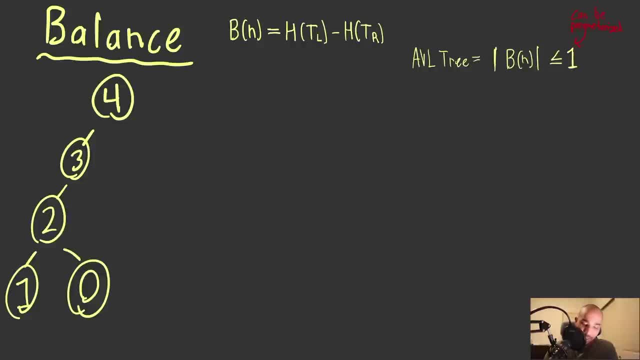 look at this tree. Okay, So we have a tree right here. Let's start at the four and let's find the balance out of four. We're going to need the left subtree minus the right subtree And that's going to give us our balance, The right subtree of four. let's do that very quickly. It's empty, So just. 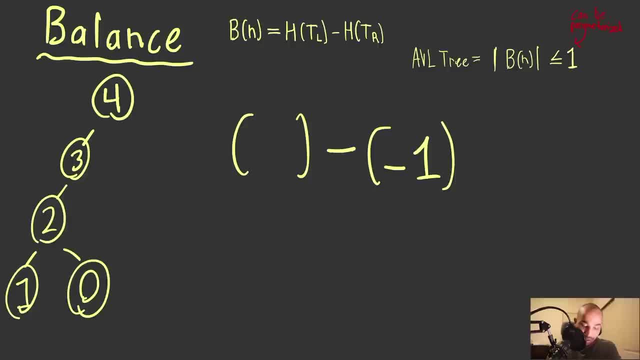 minus one, So the left subtree has a height of a height of zero, and then we have one and then two. So then we can just eyeball this and we can see the height is two. We could do the math, but we can see that we have a single node which is zero. 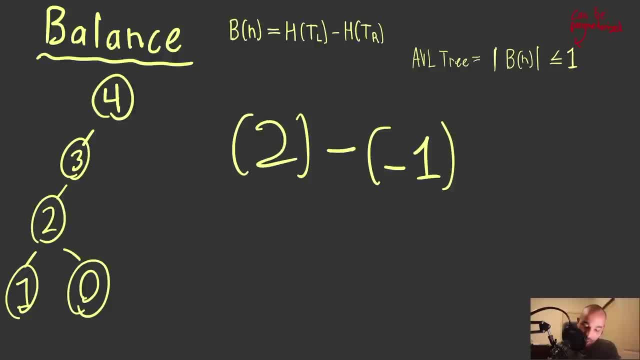 one, and then that is two minus this minus one. two plus one equals three. We see that instantly, at our root node, we have broken the property and this is not an AVL tree. So this is not an AVL tree. And this brings us to rotations. Rotations are how we're going to maintain, We're going to 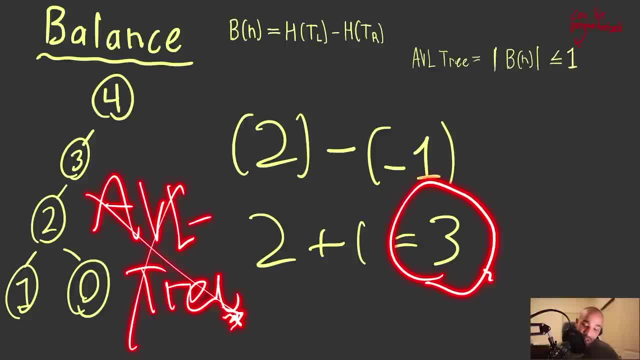 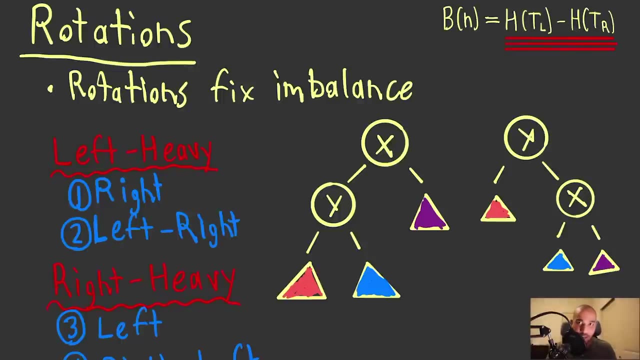 maintain the binary search tree invariant at the same time as maintaining this balance threshold. right here Let's look at what rotations are and specifically what are they trying to achieve. When we're talking about rotations, we could start out with abstract subtrees and that can get confusing if you're not used to the notation. I want to just 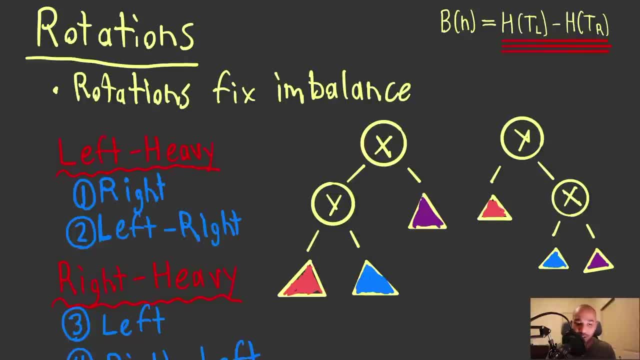 start off with some pattern recognition and just get kind of build up a intuitive sense of what should we do when a tree looks a certain way, Although in reality you would, you'd look at the math, We'll look at the implementation, but I think this is a good way to step into this first. 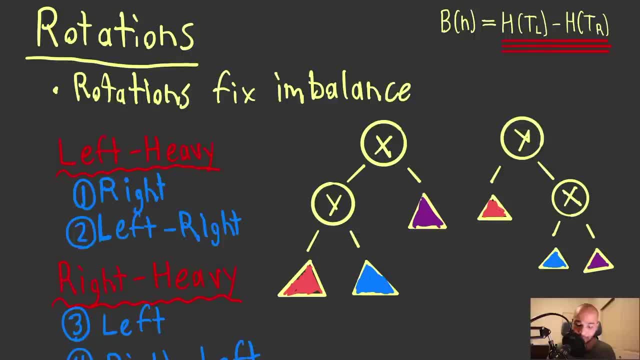 And then we'll go to the concrete implementation and it'll become very, very straightforward. Rotations fix imbalance in our tree. Basically, what we're doing, we're trying to move nodes over to the other side of the tree. that needs nodes If we're left heavy. 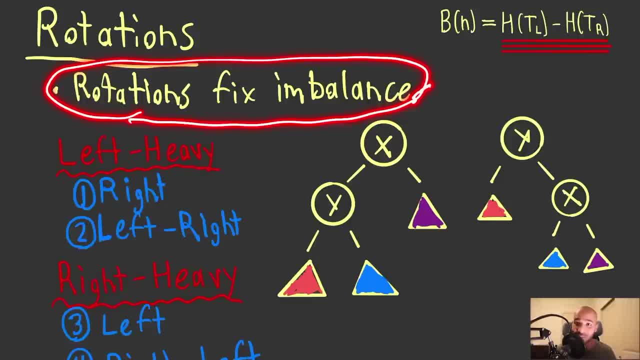 we want to go to the right. If we're right heavy, we want to move nodes to the left And there's specific ways we have to do this. So, specifically, if we're left heavy, we're going to do right, a right rotation or a left rotation and then a right rotation. We would call it a left to right. 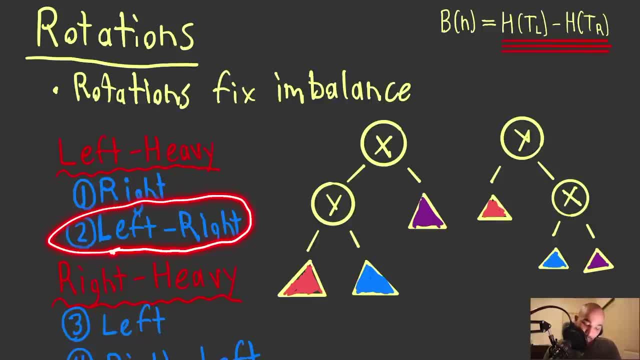 rotation And we're going to see exactly what these look like. No worry about that. If we're right heavy, we're going to throw nodes over to the left. We can do a left rotation or we'll do a right rotation first and then a left, And we'll see. these two guys are confusing at first. These 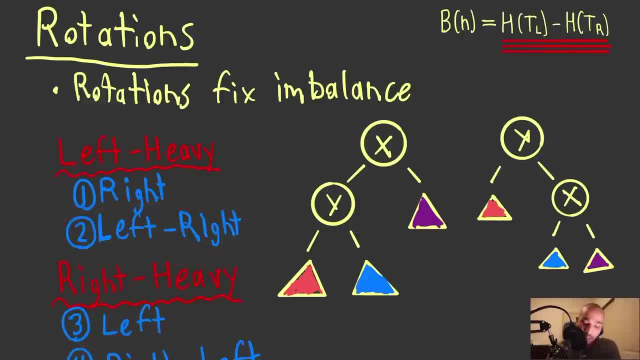 are confusing until we see examples of what they look like. Here we see a right rotation, So this guy is a right rotation And I want you to notice the tree on the left up here. it could be left and we're trying to move nodes to the right subtree. The key thing I want you to notice is: 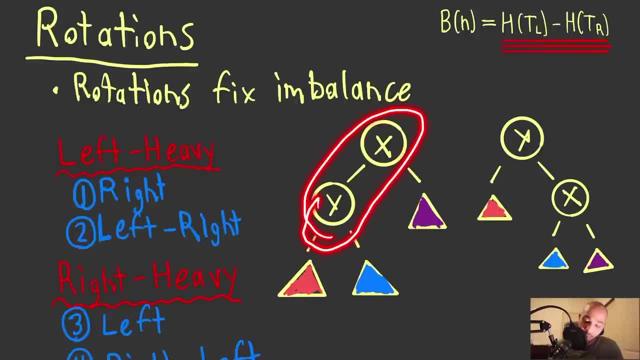 there's always two nodes in a tango. whenever we are doing these rotations, Two nodes are going to be critical and then all of the other subtrees are going to dance around and they're going to maintain that binary search tree invariant as we move these two critical nodes. Notice those X and 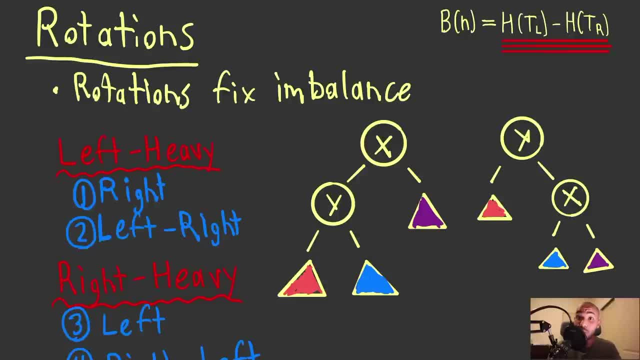 Ys. Those are the nodes we're going to care about And notice the special properties we're maintaining, doing this right rotation, And these will be clear as we do examples: There's a node X and there's a node Y. We know that Y is less than X. Let's just write some. 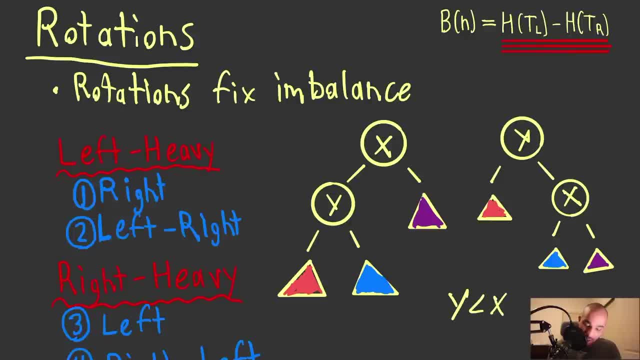 things we know. Y is less than X, So we see this little red triangle. What do we know about that red triangle? We know that that red triangle is less than Y and less than X. We're just going off what we know. We're not doing any abstract rotations, We're not making abstract subtrees. 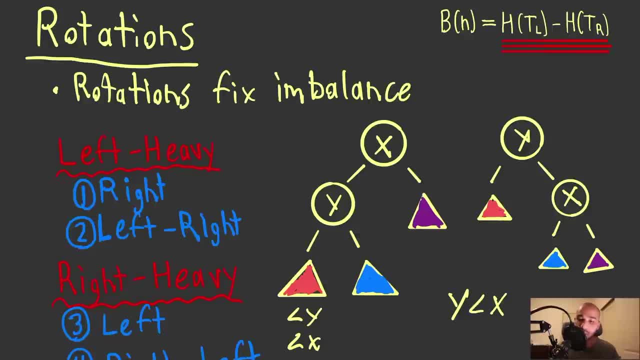 We're just looking at what the tree is telling us, And this is a really good way to reason about data structure problems. Let's look at this blue triangle. This blue triangle is greater than Y, greater than or equal to Y, and it's going to be less than X, That blue. 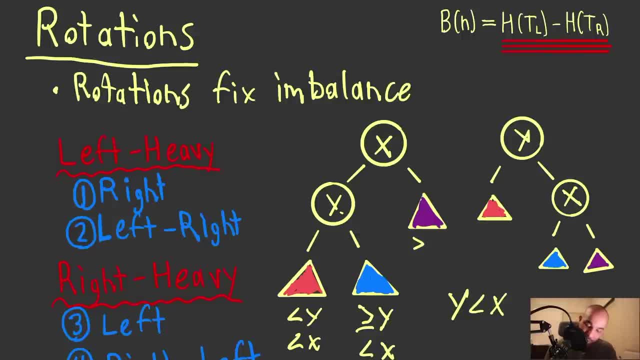 triangle fits that property. This purple triangle will be greater than or equal to Y, and it will be greater than or equal to X. What we do here is we want to move these nodes to the right. We're going to turn Y and we're going to push Y up to where X is, And then we're going to bring X down and move. 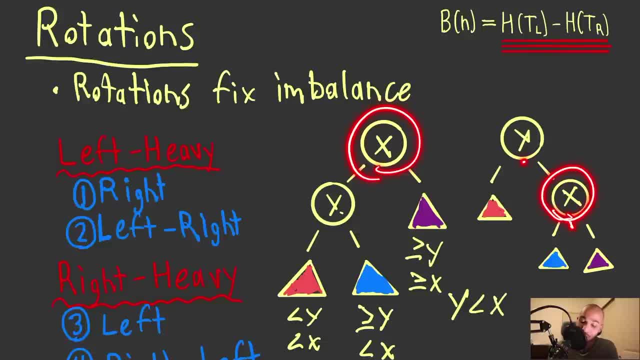 those nodes down And we're going to move these nodes down. This is theから tree. If you can see that in the window, that's going to be the right child of this Y, which has just become the root of this new tree. Forget about all of these sub trees. Forget about those sub trees down there. 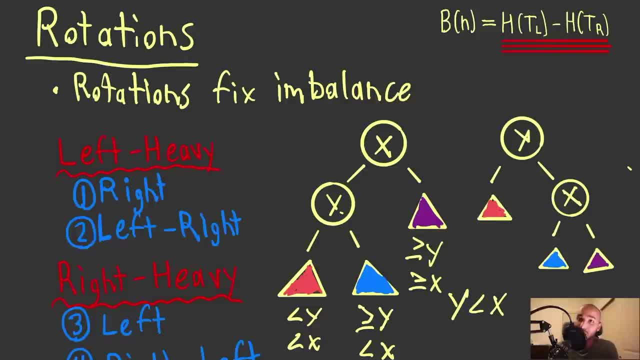 Before we do anything, I just want you to notice: Whenever we're doing rotations, just move the Y and the X. So the Y is going to move to the root, the X is going to move down. Now we need to know the subtrees fall in place So that we maintain the binary search tree invariant and we don't lose any nodes. We don't want to lose any nodes. Let's close the subtrees. 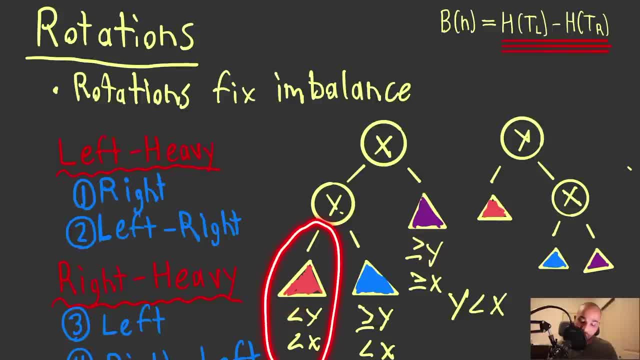 look at the properties that we had before, so we see that this subtree right here, the red one, less than y, less than x, over here, this subtree right there, that makes sense. that's also less than y and less than x, so that holds. so then let's look at this blue subtree right here, so this guy is greater. 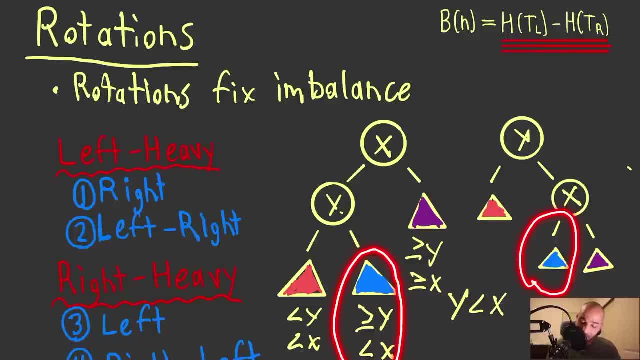 than or equal to y and less than x. and yeah, that makes sense. we went greater than or equal to y and then we went less than x. so everything's checking out. so now this purple subtree right there, we're going to go greater than or equal to y- great, we did that. and then greater than or equal. 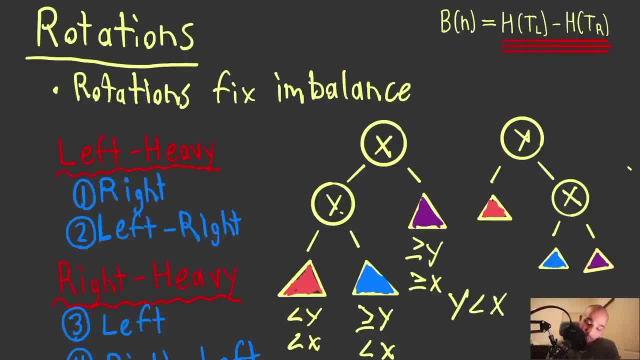 to x. so we did the same thing. and guess what we just did? we just performed a rotation of these two elements and we kept all of these subtrees, we maintained they their positioning and their ordering. so this is still a binary search tree and we have fixed the balance now that we we've seen a 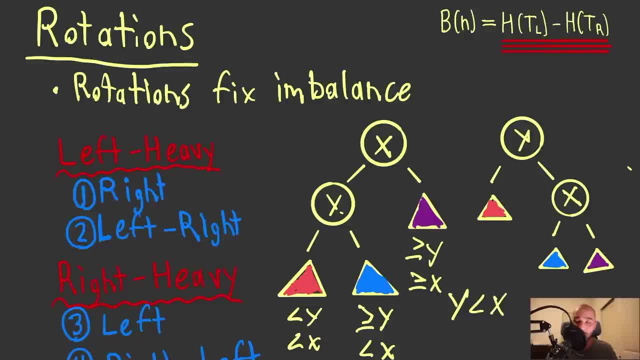 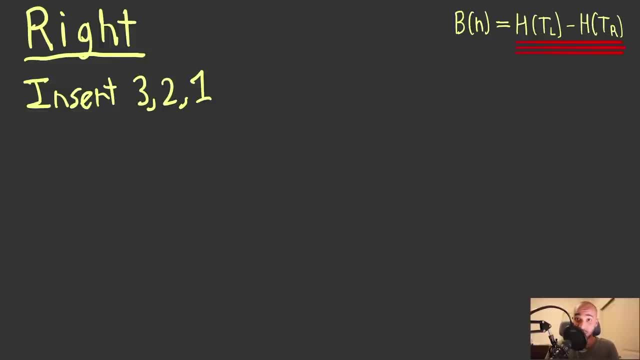 rotation in action. let's look at all the specific rotations so that we can get a better feel for it them. so remember, order matters. when we're doing insertions on binary search trees, we're going to perform these insertions. every single time we perform an insertion, we're going 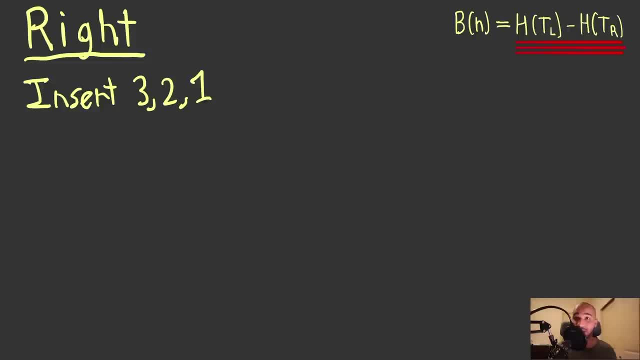 to be checking to make sure we didn't break balance at any node, break this threshold property. okay, so let's insert three. okay, we inserted three. we're gonna insert two. if we insert two, we're gonna wanna go to the left. so let's insert two. so we just inserted two. this is still a binary search. 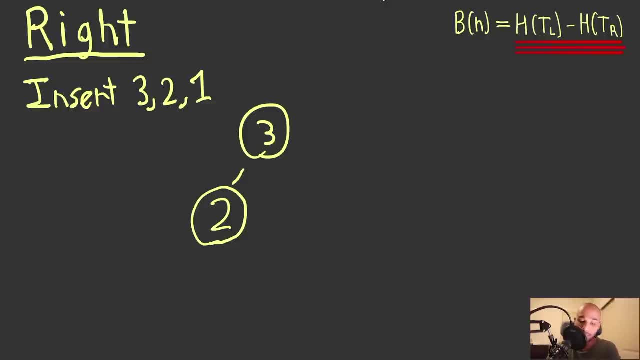 tree, all of the balances, check out and we could recalculate them, but for the sake of time, um, i'm just going to. you can do that in your head. we'll just continue with this demonstration. now we're going to need to insert the one, so we're going to go to the left and then we're going to go to. 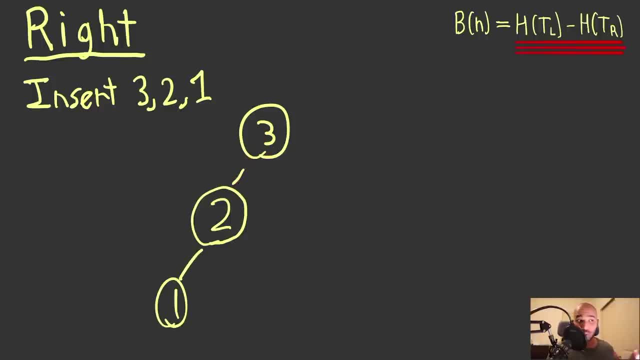 the left, but there's a problem, and so the more of these that you do, you're just going to be able to see it. i don't want to do the math at every node, eventually just going to be able to see whether there's an imbalance. but in reality, if you were coding this, you would want to know concretely. we're. 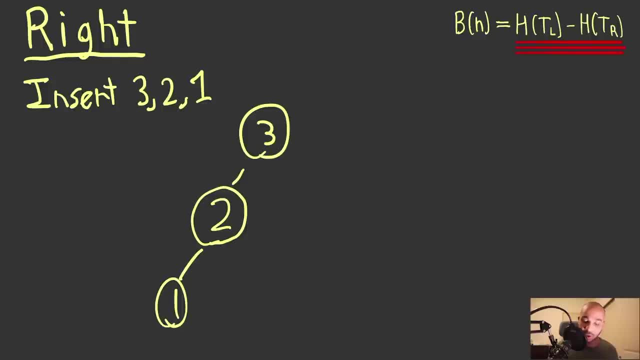 going to be recursively after this: after this node gets inserted, the call stack will return to this function call and then we're going to be able to see if there's an imbalance, or if there's an imbalance, and then we're going to check the code, and then we're going to check the code, and then 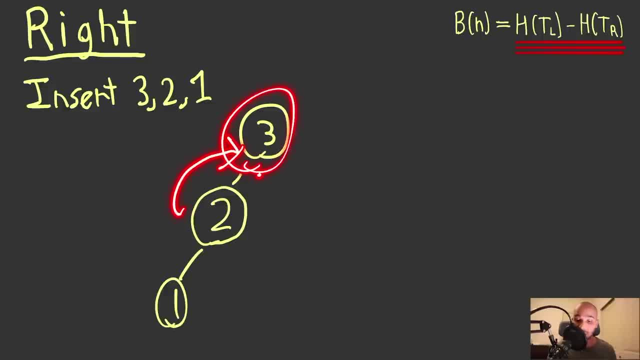 he returns, he's going to check his balance. that's how it would actually be implemented. but for the sake of um- just you know speed- we're just not going to trace it, as the code would do it, we're going to just talk it through. the root is imbalanced. we have the. the right is minus one. 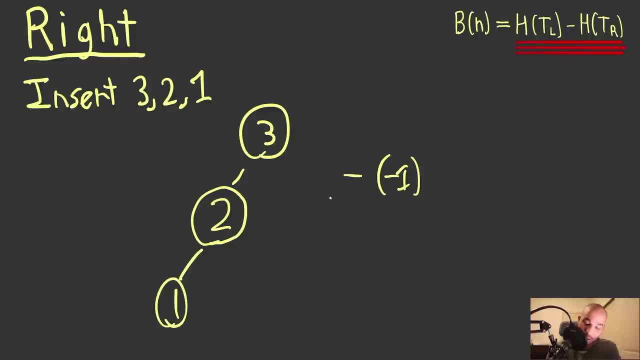 and then the left is going to be a depth of one, so this leads to a two. so this is bad. we just broke the property, and so what rotation can we use? notice what our balance is. our balance is two. and remember, since our balance is two, the left guy, the left subtree, is dominating. we are left. 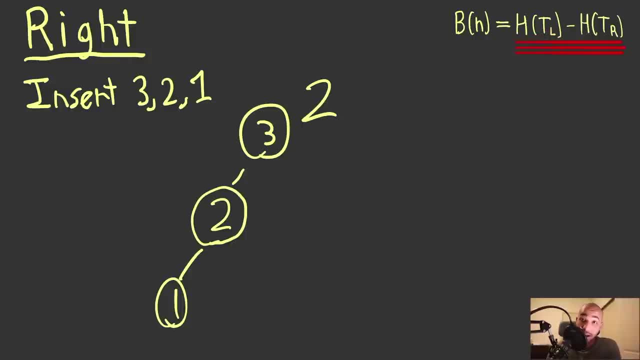 heavy. so what does that mean? we can do? a um, a right rotation, get those nodes out of the left subtree, move them to the right, and so there's. there's a catch to this. we'll see that when we get to the left right rotation, which is next. so remember, when we do the rotation, only focus. 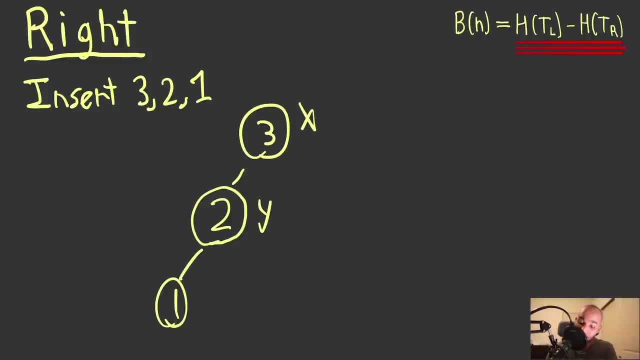 on x and y only focus on two nodes. we're going to move this two up. we're going to move the three down. we need to fix the subtrees. remember, there's actually three subtrees. uh, going on, going on. here we're going to have this subtree, we're going to have this subtree. 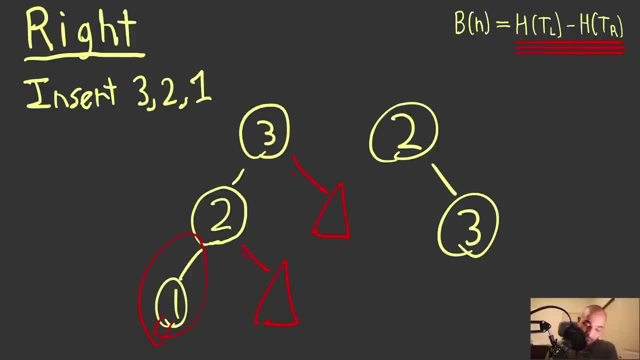 and we're going to have that subtree. what do we do with those? so, first off, these guys don't even exist. so they, they don't even they're, they're not even in the picture. the code would have to handle them if they were populated. but this one, where does that one go? well, we know, one is less than. 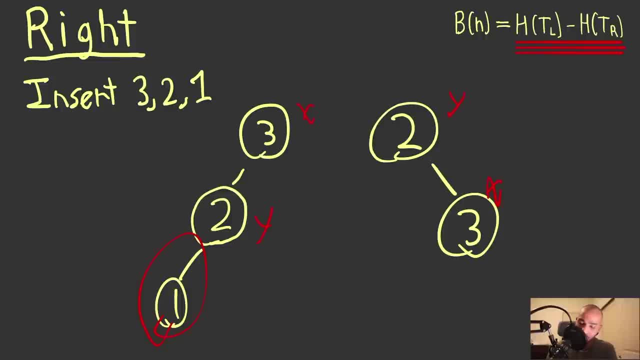 this y. we know one is less than the other one, so we're going to move this one up. we're going to move this x, so this one is: can this one can just go here? um, this is less than y, less than x, so we've maintained our property. so that is the right rotation. completed. notice how we started out. 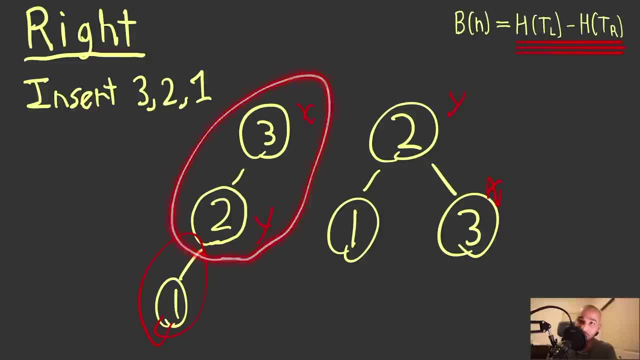 we just rotated these guys. just worry about x and y. just rotate the nodes that matter and then adjust the subtrees. we saw that this subtree gets adjusted. that is the right rotation. take these guys, move them to the right. we're rotating to the right, so now we can see that we're left heavy. we fixed the left heavy by moving to the right, so now let's. 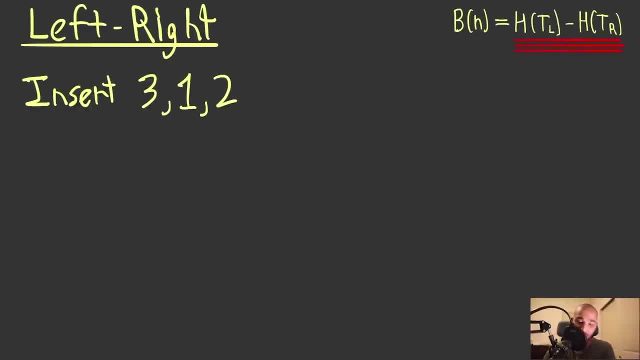 look at a different situation where we're left heavy but we can't just do the right rotation. so now we're at a left right rotation. let's do this: let's insert the three, then we insert the one. we can eyeball this. we still see that we're balanced. and then we insert the two, we're left. 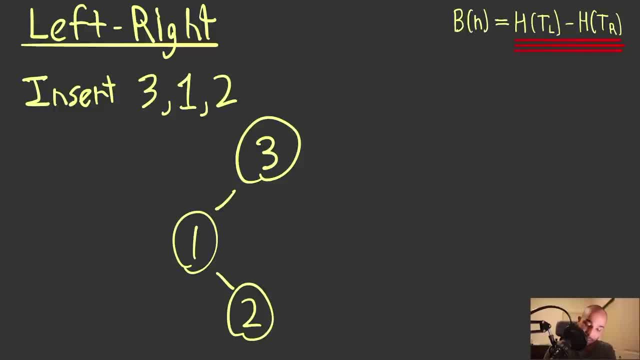 heavy. if we calculate the balance at the root node, which is where balance is broken, we're going to see that we have minus one in the right subtree and then we're going to see we have a balance of one in the left. so again we have a balance of two. can we just do the right rotation? we're going to 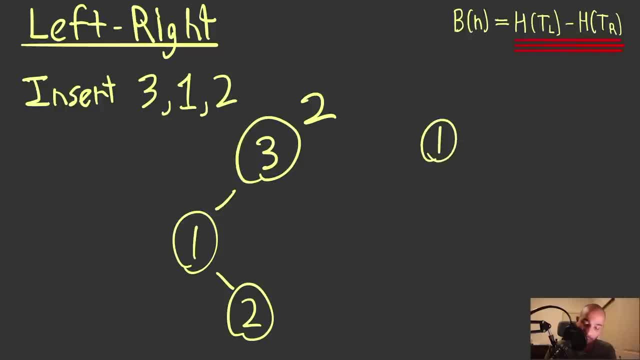 try that. let's just try doing the right rotation: pull the one up, push the three down. that is the right rotation. started and then the two. the two is gonna have to go right there because it's greater than one in less than three. it's greater than one in less than three. 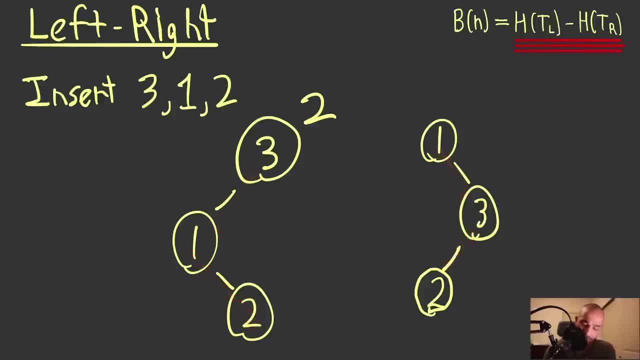 it's greater than one in less than three. but this is not balanced. if we look at the root, the root has a minus, one minus. if we look at the right, this has a balance of one. this is minus two. this is not balanced. this breaks the avl property. so we can't just do a. 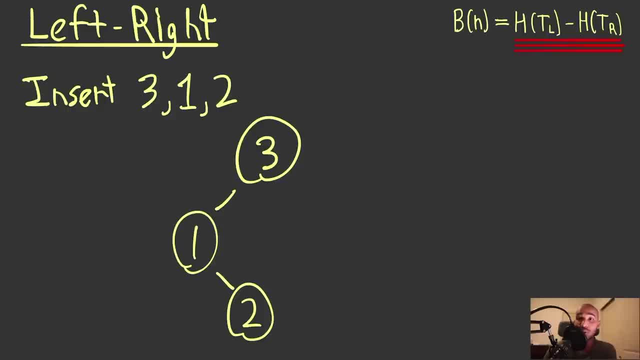 right rotation. here there's something different we have to do. this is where we would do something called a left right rotation. we're going to take these two guys right here, these two guys, we're going to do a left rotation and then, once we do a left rotation there, we're going to do: 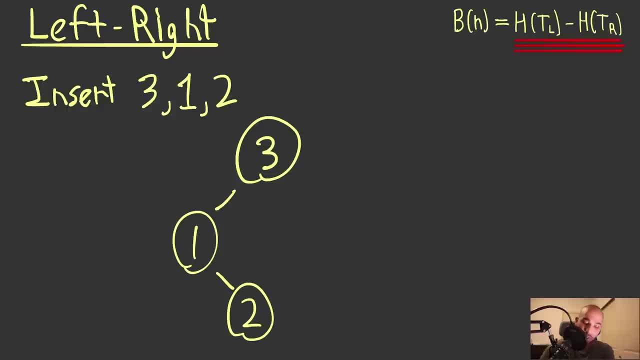 a right rotation on the subsequent node. so first let's do a left rotation. so we're gonna pop over the two, pop over the one. so we did a left rotation there and the three is just going to be up here now we've performed the left rotation right there. that's the left rotation. 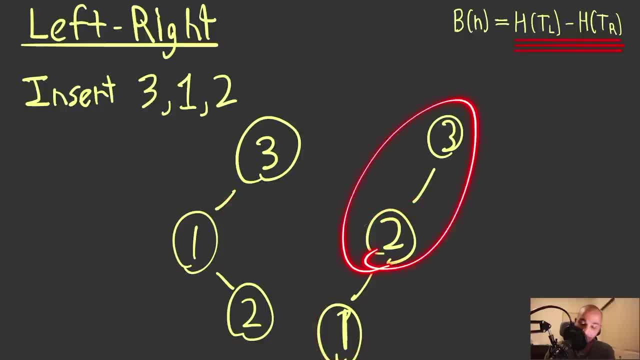 and so now we need to perform the right rotation up here. so we're going to do the right rotation, so now we're going to push the two up and then the three down, and then the one goes here. so this is it, this is the final tree, and this is a balanced- uh- binary search tree within our threshold. so that's. 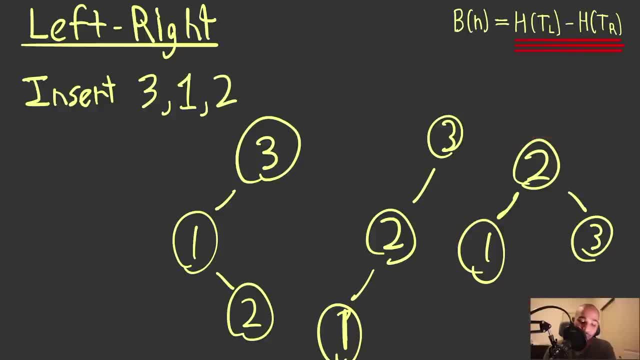 left to right. both of these are left heavy restorations. now that we understand how these rotations are done- or at least we saw initial examples- we can look at how we fix right heaviness. and it's the exact. it's just the opposite. it's the same operations. so now let's insert one. let's. 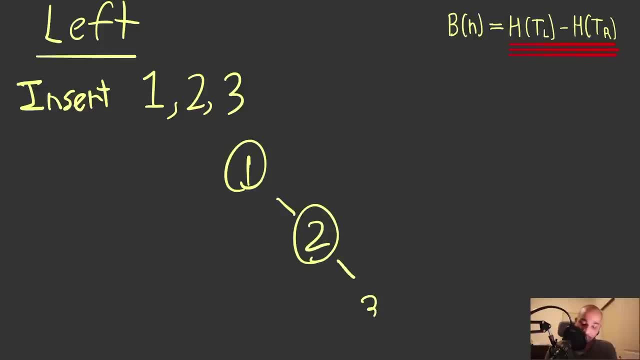 insert two and then let's insert three. we see we have a problem and now we can do a left rotation, so we're going to bring the two up, we're going to bring the one down. so, remember, these are our nodes we're focusing on and we're moving to the left so that that one moves to the left. 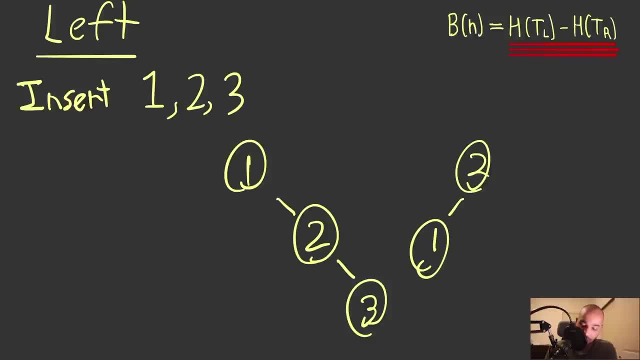 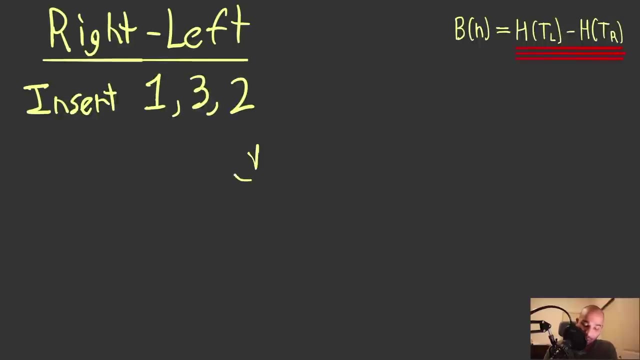 because it's a left rotation. and then this three just goes right there, and then this is our- uh, finished binary search tree. so choose the root, left, right, and that is the tree. so that's our left rotation. and then let's look at right, left, so insert a one, we're. 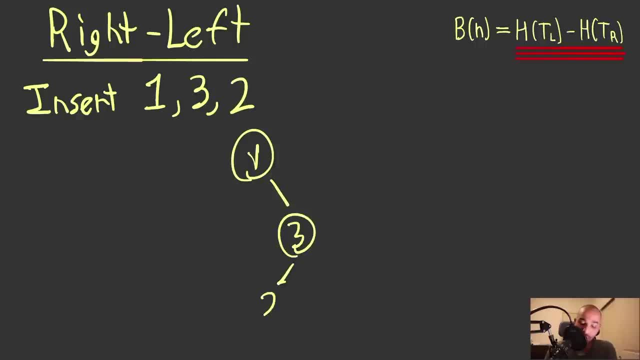 going to insert a three and then we're going to insert a two, and this is when the balance is broken. but again, if we just do a left rotation, what happens? we're going to see three, we're going to have a one there and then the two is just. the two is greater than one. less than three, um greater.